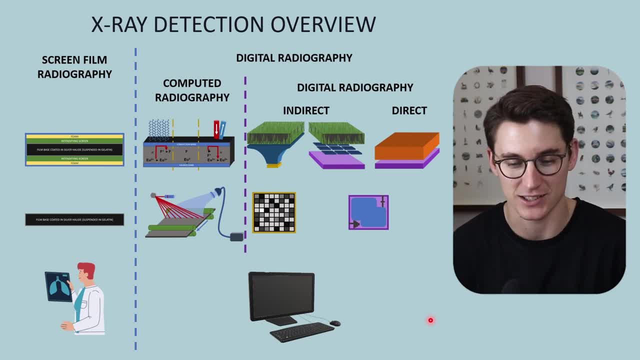 in order to generate a radiograph that we will end up looking at and analyzing Now. x-ray detection systems detect x-rays that have been transmitted or scattered through a patient and convert that x-ray signal into an actual radiograph. Now we can broadly classify. 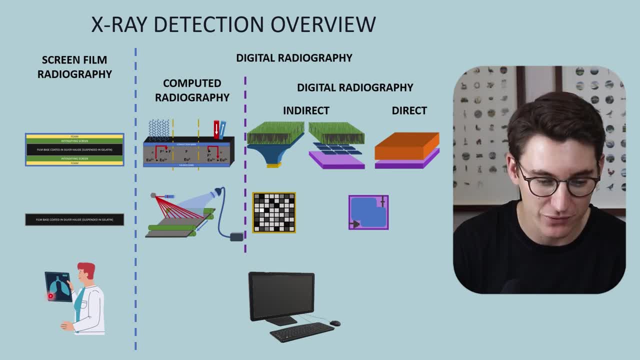 x-ray detection systems into two main categories: screen film radiography and digital radiography. Now, when we talk about screen film radiography, we are talking about the actual plastic film that we hold up to a light box, and that film has varying, different optical densities, allowing different 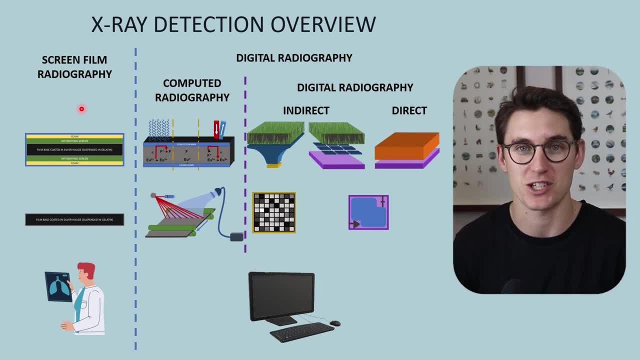 amounts of light through the film and creating the radiographic image that we see on the film. Now, this film cannot be manipulated digitally. It's not on a computer screen, It's a physical copy that we can carry around. Digital radiography systems refer to the digital image that we are. 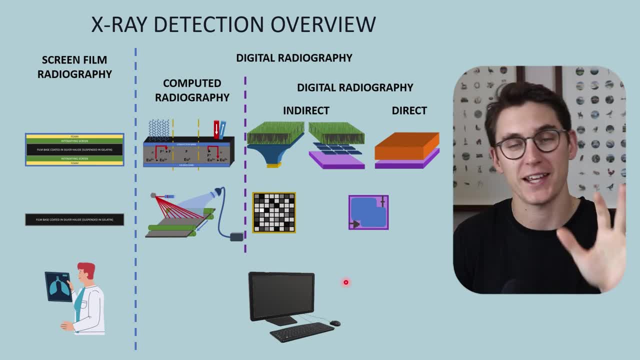 creating The final radiograph will be available on a computer screen. That computer screen, that radiograph, will have pixel values for each one of the pixels in that image and because those pixels have a grayscale value, we can manipulate that image. after we've taken the image We can. 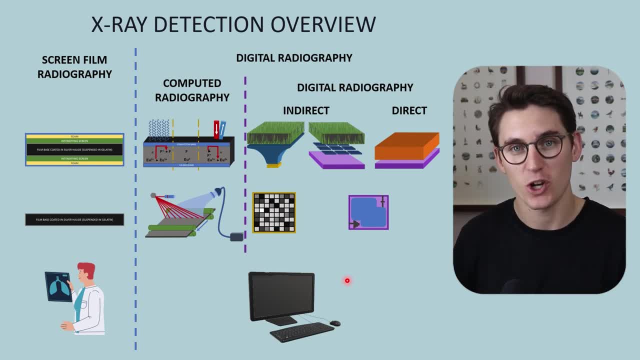 increase the quality of the image. We can increase the quality of the image, We can increase the contrast, we can increase the exposure to the image, we can digitally manipulate that image. Now we can further subdivide digital radiography into two separate categories, and this is where 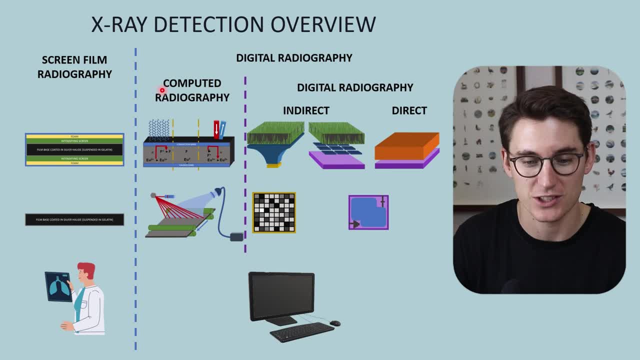 it sometimes gets a little bit confusing. The first category is known as computed radiography and the second is called digital radiography. Now, this initial digital radiography is referring to the end product, a digital image. This second classification, digital radiography, refers to: 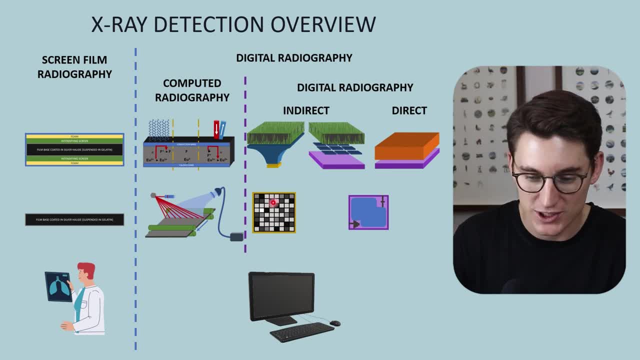 the way we process and store our image. The processing and storage of the x-ray images here in digital radiography happens in a digital manner. We are storing charging capacitors that can then be transferred to a computer. In computed radiography we create a latent image. 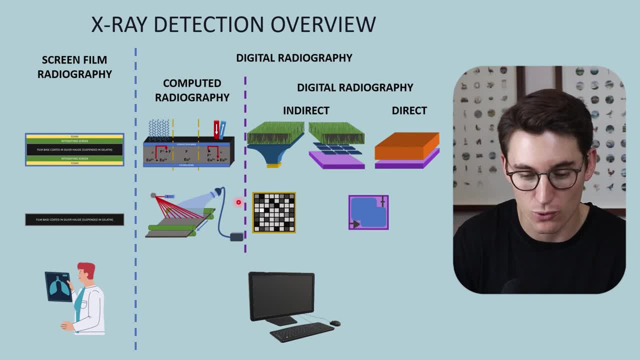 in our computed radiography cassette that we can then process into a digital image. This is a manual process: the processing of this image that then converts this latent image into a digital image. This is a manual process: the processing of this image- that then converts this latent image into a digital image. 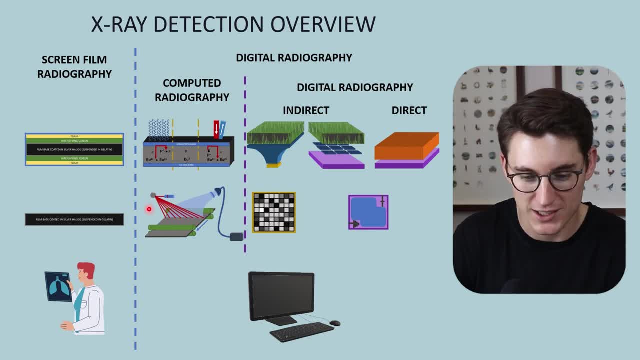 So the processing, the storage of the images in computed radiography is analog and in digital radiography is digital. Now we can further subdivide x-ray detection systems into cassette-based systems and cassette-less systems. Both screen film radiography and computed radiography require us to hold a cassette that we 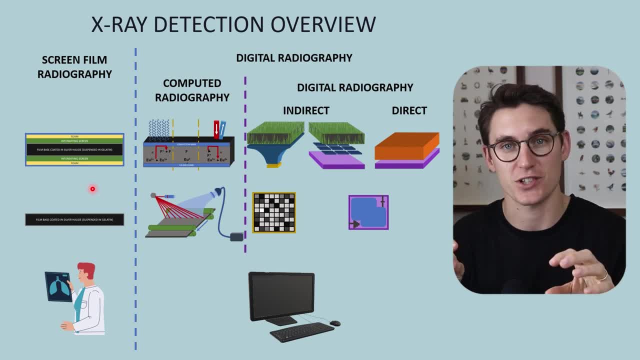 then place behind a patient and once we've exposed that patient to x-rays, we can physically take that cassette away for processing in order to create our image. We don't get the image instantaneously on our computer screen. That cassette needs to be opened up, needs to be read out, and then we can. 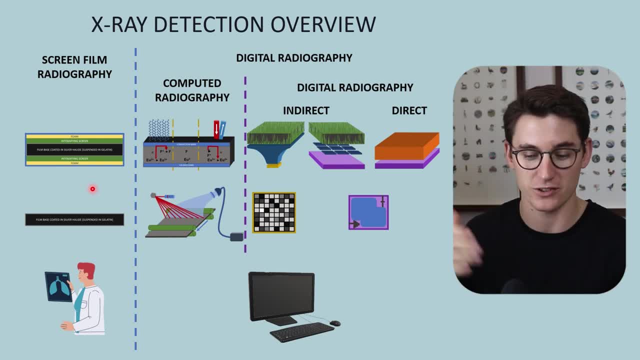 create an image, be it a film that we can physically hold or a digital image that we've sent to our computer. in computed radiography, In cassette-less systems, we can get an image almost instantaneously sent to our computer. Everything is digital in that pathway. We don't need a physical cassette. 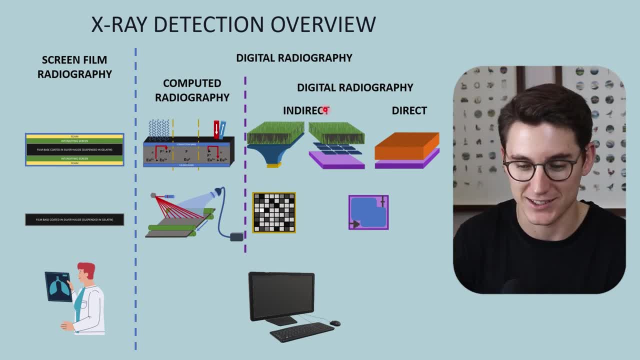 that we take and process In computed radiography. we don't need a physical cassette that we take and process. We can also subdivide these systems into those that require scintillation and those that don't. Now, scintillation is the process of converting x-ray energy into light, and that light energy is 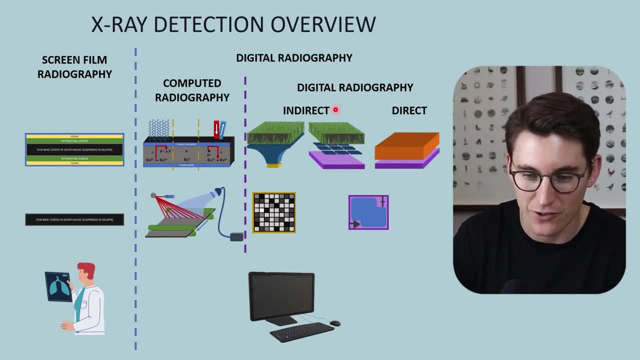 then used to create our x-ray image. So our indirect digital radiography system and our screen film radiography system both require scintillation. Computed radiography and direct digital radiography do not require scintillation. Now, this scintillator layer here. 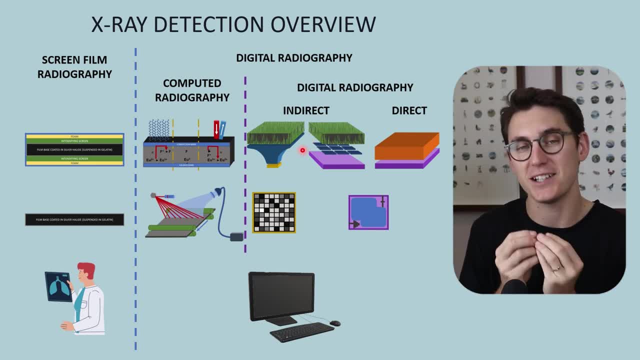 we're going to look at, and the process of fluorescence- immediately converting x-rays into light- is a process we're going to look at. There's another process here called phosphorescence, where our x-ray energy is then later converted into light, and when there's a delay in conversion, 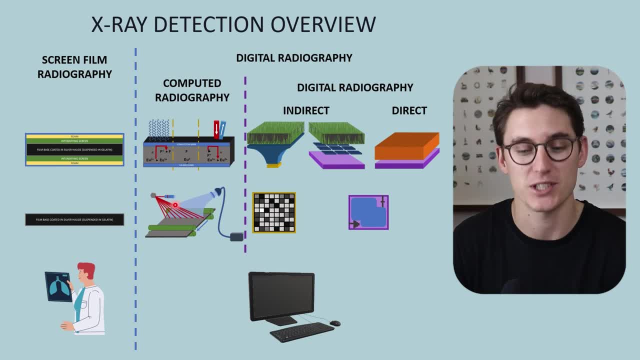 of x-rays to light. we call it phosphorescence, Again a process that we will look at when we look at computed radiography. So it's good to know, when we take a step back, that there are multiple different systems. We've got a screen film radiography system, a computer radiography system and a screen film radiography system. 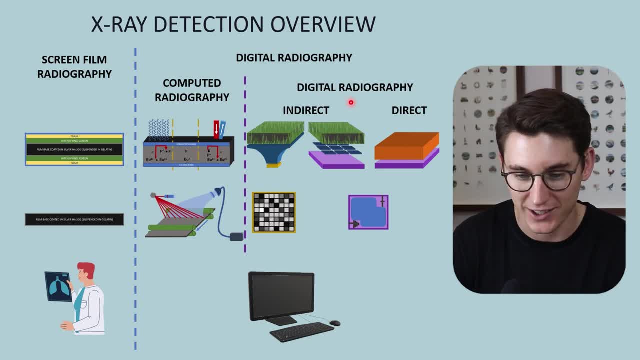 We've got a screen film radiography system, a computer radiography system and a computer radiography system. We've got a screen film radiography system, a computer radiography system and a screen film radiography system, Our indirect digital radiography system, which can either be using a CCD chip or a TFT array.